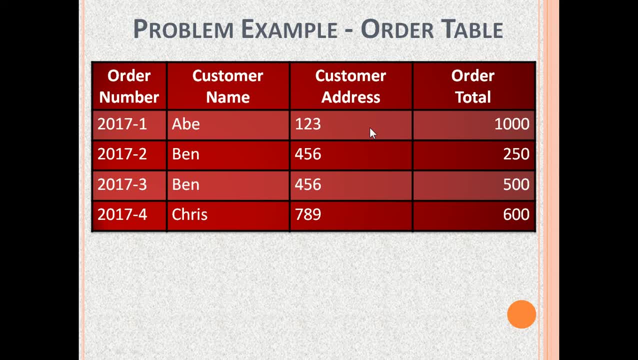 This gives rise to issues. For example, if a customer's address changes, some rows may be updated with the new address and other rows may still have the old address. To continue, we will see the table with the new address. To continue, we will see the table with the new address. 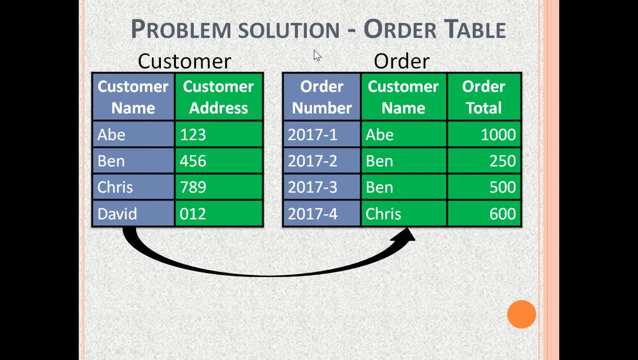 To continue, we will see the table with the new address. To convert the order table to 2NF, it needs to be broken into two tables: Customer table with columns, customer name and customer address. Customer name is the only candidate key and customer address depends on it. 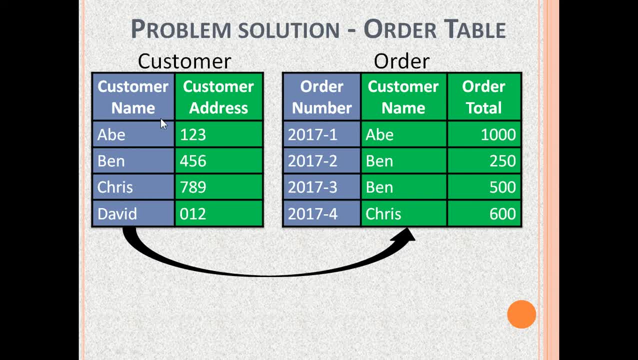 So this table is in 2NF. Later, if we get duplicate customer names, we can make customer name and customer address together as a primary key. This is the order table with columns OrderNumber, CustomerName and OrderTotal. OrderNumber is the only candidate key. 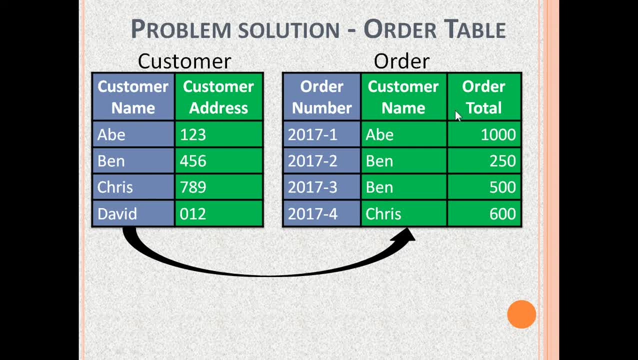 CustomerName depends on OrderNumber. OrderTotal also depends on OrderNumber. Once these tables are in 2NF, the issues are resolved. Every customer's address exists in a single place and can be updated there. By the way, CustomerName in CustomerTable is the primary key. 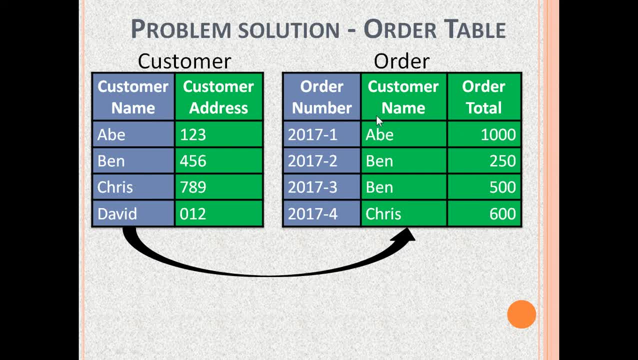 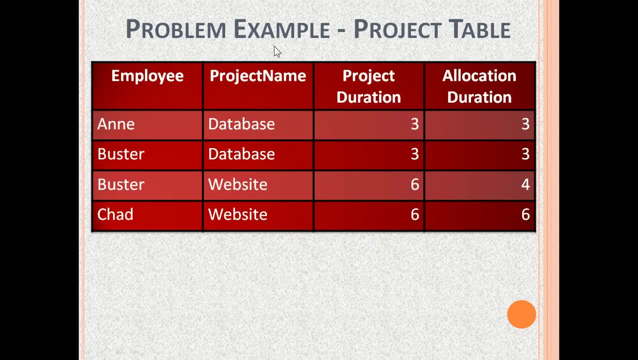 CustomerName in the OrderTable is called the foreign key, which means it is the primary key of some other table. Another example of a table that is not in 2NF: This is the project table with columns Employee, ProjectName, ProjectDuration and AllocationDuration. 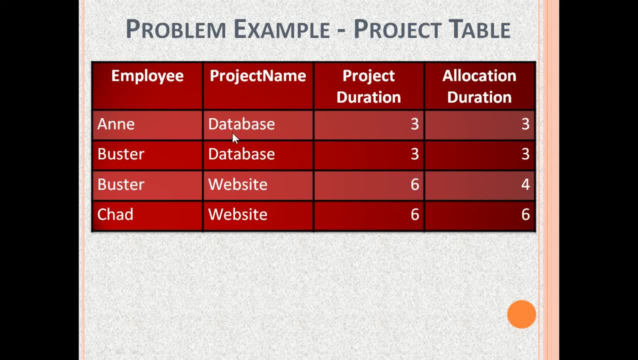 For example, Annie is in Database project whose duration is 3 months and her allocation is also for 3 months. Now, a project may have one or more employees allocated to it. For example, both Annie and Buster are allocated to the database project. 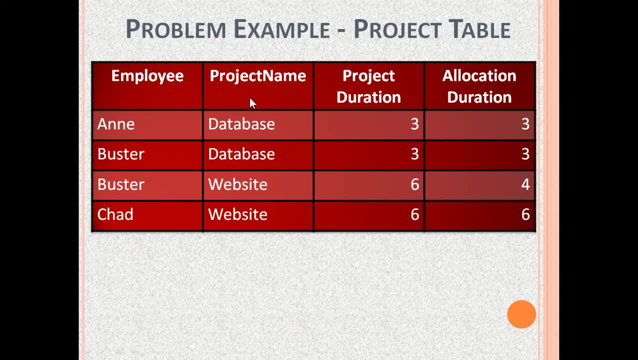 ProjectName is not a candidate key because multiple rows have the same project name. These two rows have database as a project name. These two rows have website as a project name. An employee can be allocated to multiple projects. For example, Buster is in both.